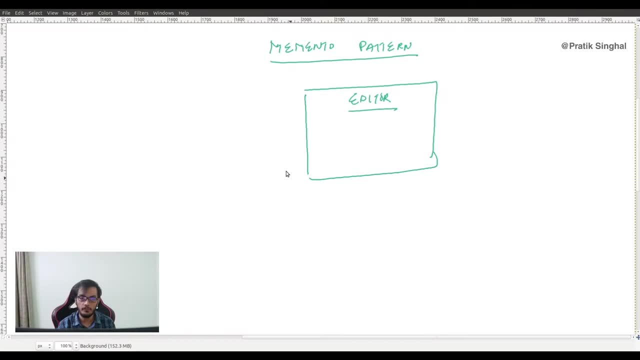 click on undo and now you want your editor to restore to its previous state. Now here to represent an editor. we have an editor class right Now. this editor class can contain data, like it can contain text. it can contain data like cursor position. it can contain any formatting that. 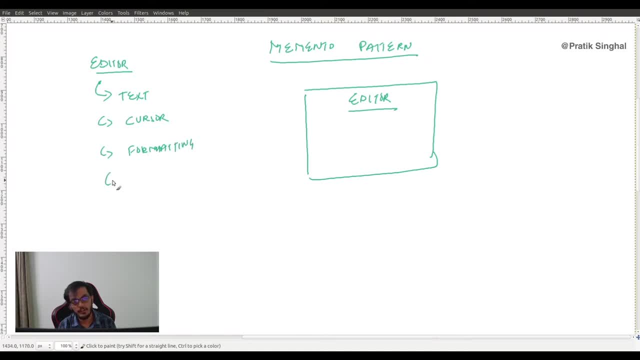 you have applied any settings that you have stored here. So a lot of things are there in this editor. Now, when you want to, let's say you are typing something or you do make any change- let's say you change the settings. right, We need to create a snapshot of the editor state so that 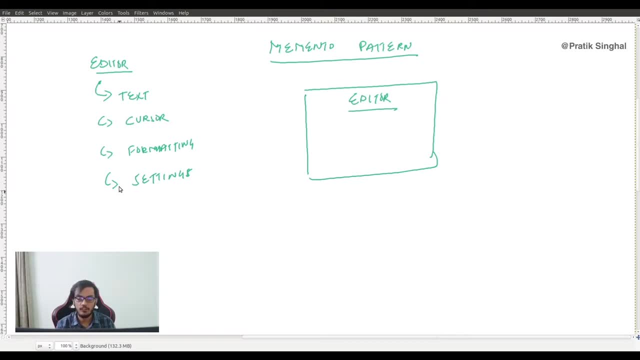 we can later on undo it, Like let's say for example, in the settings let's say, zoom level is mentioned. So let's say, right now the zoom level is 100% and you change the zoom level from 100% to 120% right Now, if my editor has to support fully the undo functionality, then the editor 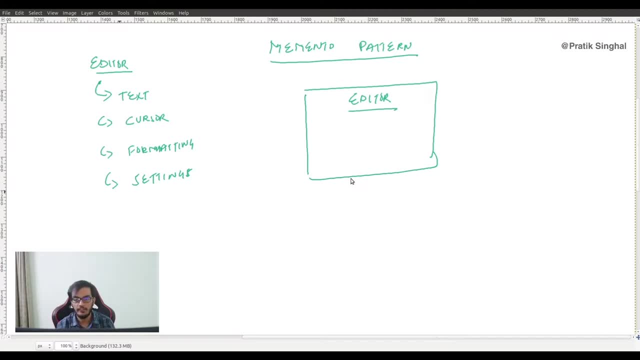 state that was there, right, the snapshot, or the data that is there in the editor. I need to save it in some place, right? At least I need to get access to that state from some place right Now so that in the previous state I will show that, okay, zoom level was 100% inside the settings and 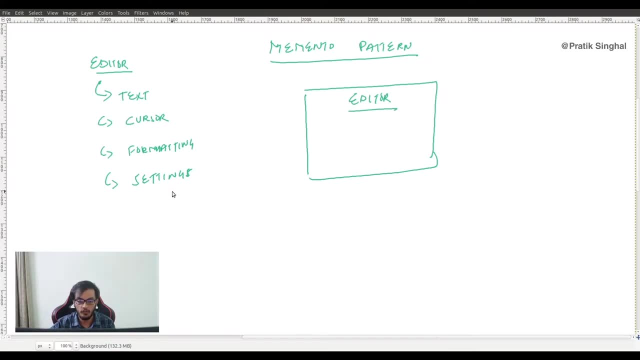 later on, when, when the zoom level reaches 120%, let's say, you press control plus, that you want to undo it, then I know. I know that. okay, there is a previous state to which I can restore my editor state or editor data right Now. the problem is: how do I create this state? 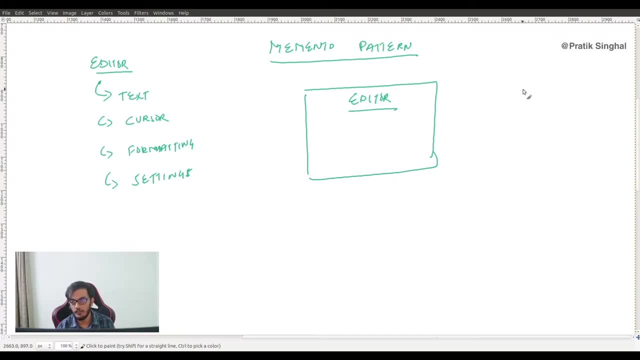 So let's say, for example, I create another class- let's call it the class as helper class, and this helper class wants to create a snapshot of the editor class right Now. the problem that we will face when the helper class wants to create a snapshot of the editor classes: 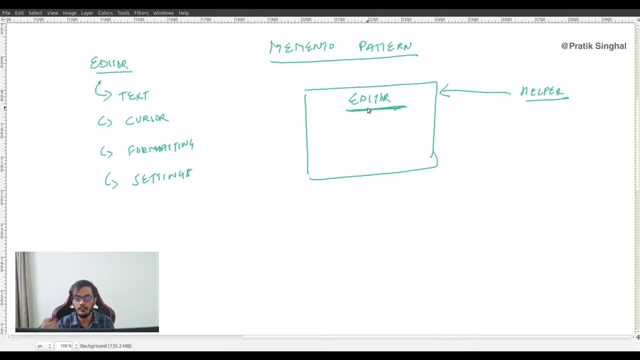 that this helper class will need access to the editor classes internal state. it would need access to in the editor classes internal data that it is maintaining right which may not be possible to give because of encapsulation. maybe editor class has some private variables which it can, which it does. 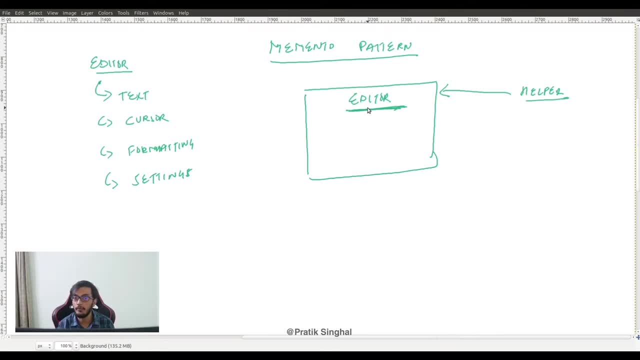 not want to give access to the helper class right. So in that case, how will helper class make the state? It's not simply possible to make the state right. Another thing is that even if, let's say, I make all the variables inside the editor classes public, that may not be a good idea because in 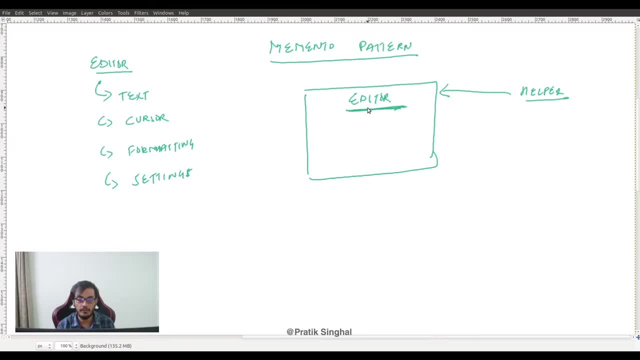 that case you are breaking our encapsulation. you are not hiding the relevant data right. So again it's a problem. so the idea behind the memento pattern is that in the memento pattern we will give the responsibility of creating the snapshot and restoring from that snapshot. 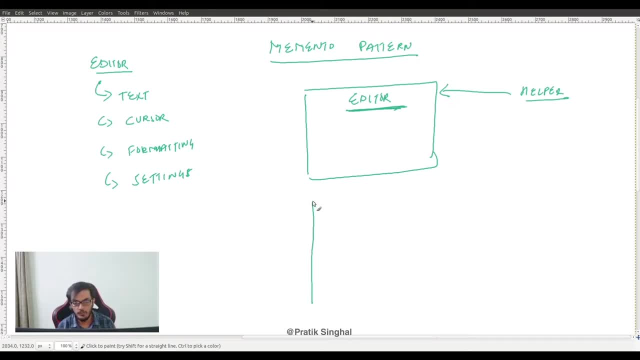 to the editor class itself. okay, In fact, what I'm going to do inside the editor class. this is my editor class inside the editor class. Since all, almost all the languages support nested class feature, or java also support nested class feature, inside the editor class, I will create a memento. so inside the editor, I have different. 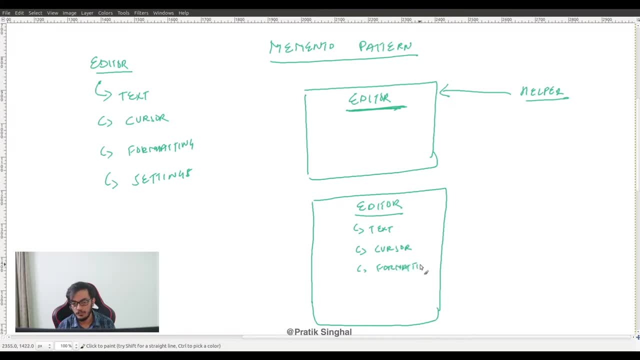 fields, text, cursor, formatting and so on, settings. now what I will do inside the editor class, I will create a memento class. okay, memento is basically nothing, but it's like a snapshot. so let's say that now this snapshot will replicate exactly what is there in the editor. so it will 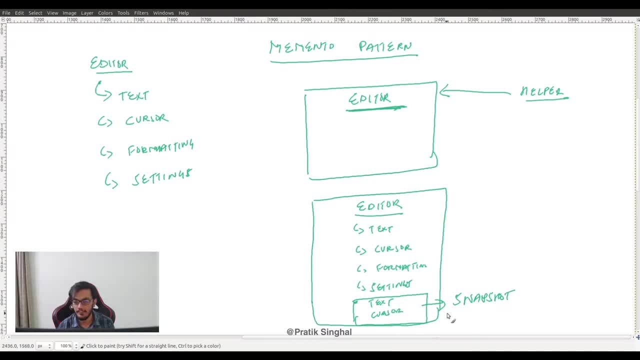 replicate text, it will replicate cursor, it will replicate formatting settings and everything right. the difference would be that only the editor class can modify this snapshot. The helper class, which I'm going to create later on. it will not be able to modify the snapshot, it can only get the snapshot. 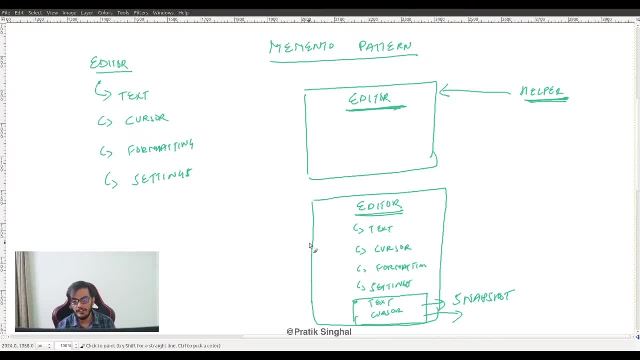 okay. so it's not breaking the encapsulation, because now a editor method will provide, can provide some, let's say, create snapshot okay, which can then, uh, provide the snapshot object. so now the responsibility of creating the snapshot is with the editor class, not with the helper class. so that's why helper 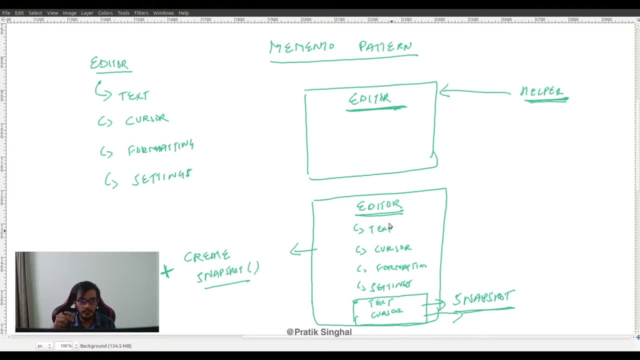 class does not need access to all the private variables. second thing is: helper class cannot even accidentally modify the snapshot. why? because all the variables inside the snapshot will be public and i will be private and i will only expose the getter methods from inside the snapshot. okay, so that is the idea behind the memento pattern. so in the next section let's look at: 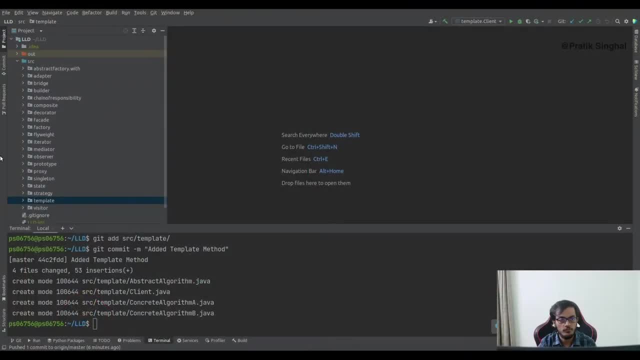 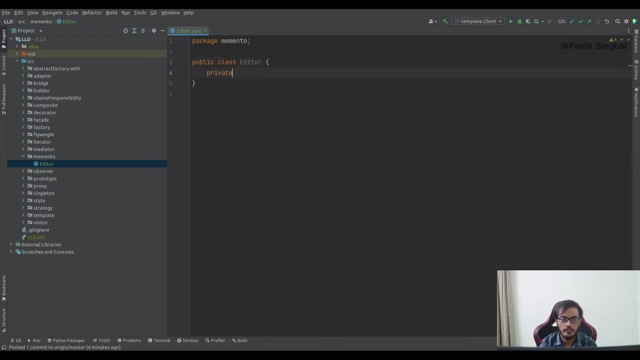 the implementation of this. let's go to our editor now. so what i'm going to do here, i'm going to create a package called as memento. now, in this memento, i'm going to create a new class called as editors. now this editor, let's say, has few private methods like text. 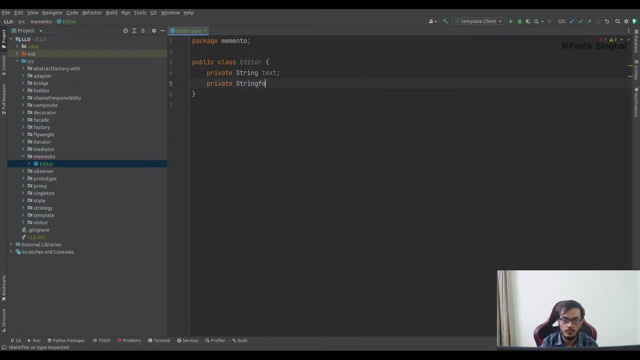 so i'm going to create a new class called as memento. okay formatting options: cursor x, cursor y. right? so cursor x and cursor y is basically the position of the cursor. now i'm going to create a constructor here and i'm also going to create a getter setup. 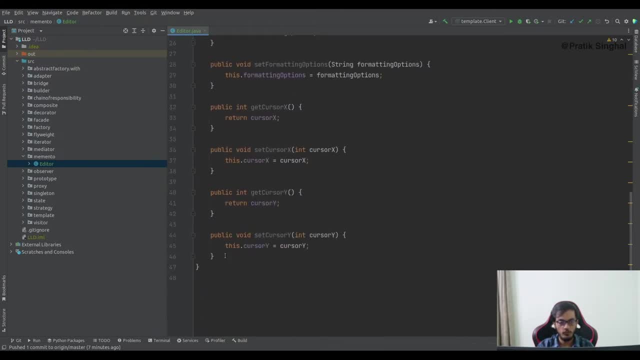 now what i'll do inside this editor also class. also, i'm going to create one nested class. let's call it the snapshot editor snapshot. now, this editor snapshot class will replicate this exact same state. okay, text formatting options: cursor x, cursor y, so basically whatever state i have. 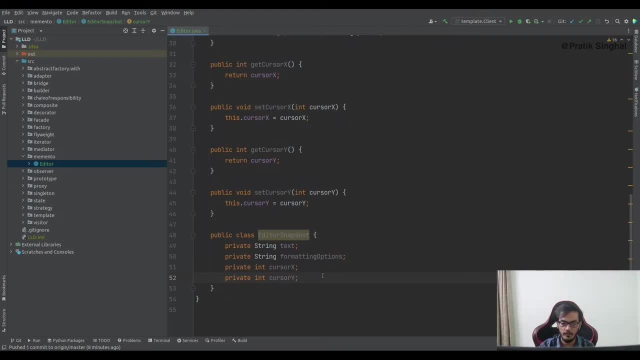 inside the editor, exact same clone i have to maintain in the editor snapshot class. now, in this editor snapshot class, i will create a constructor and i will also create some getters. i will not create any setup. i will not create any setup. okay, because the only person, the only class which should be able to call this constructor is the. 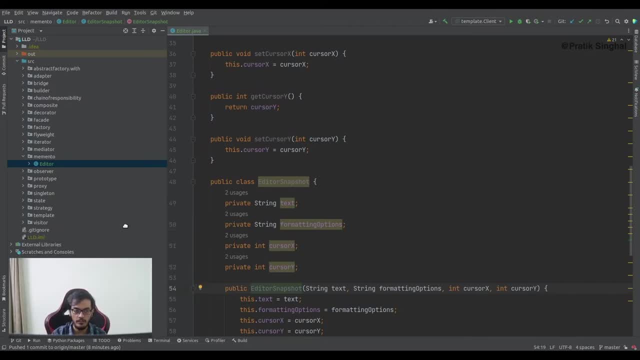 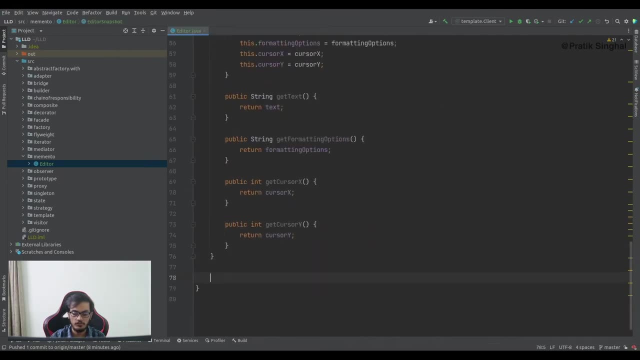 editor is the editor class right, because that editor class itself is responsible for creating the snapshot. now, inside the editor class, i will provide one method called as create snapchat, which will create the editor snapshot and and use it. so it will say: it's dot now in this editor snapshot. i will also maintain the editor state as well. okay, editor. 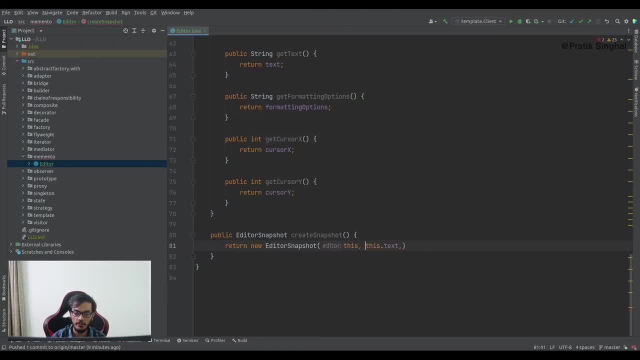 now when, when you create an editor snapshot, i will pass my current editor state. it's text, then it's formatting options, it's cursor position x, then it's cursor position y and so on. basically, whatever state, i am maintaining the returns- all that data i have to pass in the 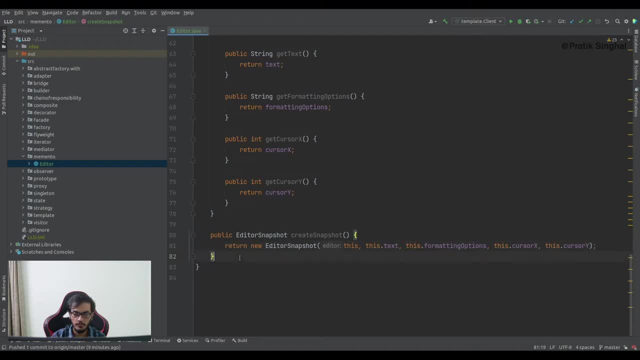 editor snapshot. okay, so this will return my editor snapshot. okay, so this is the code for uh, creating it. now. inside the snapshot, i will have a method for restoring the contents of the editor. i will just populate void restore now to restore what happens. this, whatever is this editor that i have passed here. 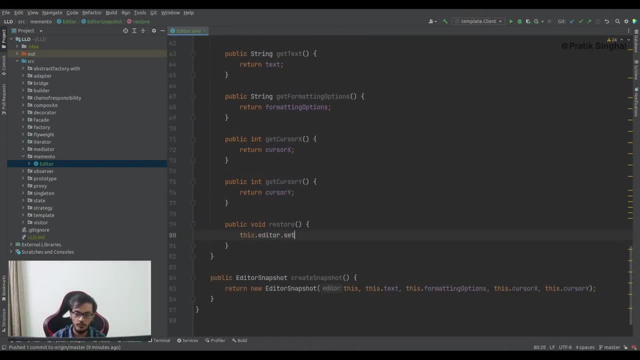 i. i will use its setup to restore the script. i will say this dot editor dot set text. whatever is the text inside the snapshot: this dot editor dot set cursor x. this dot cursor x. this dot editor dot set cursor y. this dot cursor y. it's dot editor dot set. formatting options. 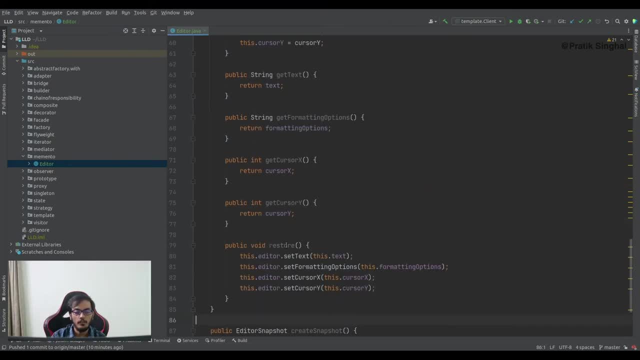 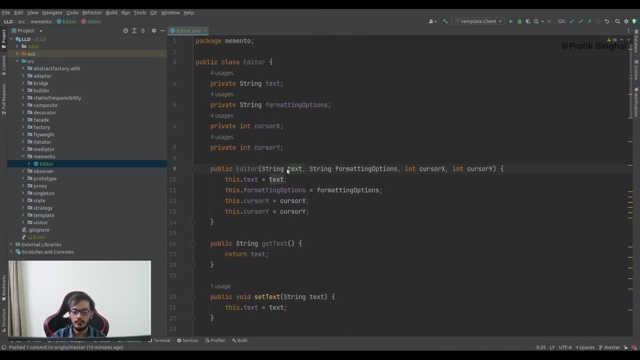 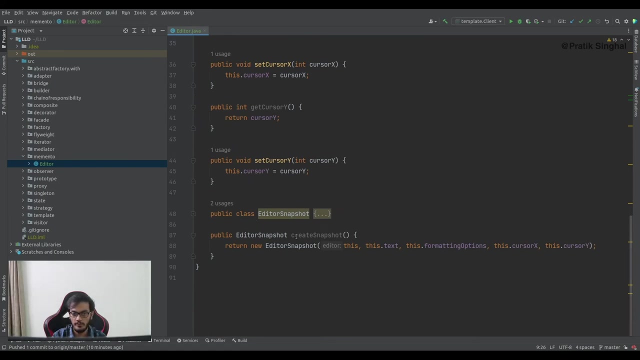 this dot automatic options. okay, so now anybody who wants to restore or anybody who wants to create a snapshot of this editor, he can- uh, they can just, you know, use these editor classes, create snapshot method. so let me just close this class now so they can use this editor classes create snapshot method to create a snapshot and for this editor, snapshot. 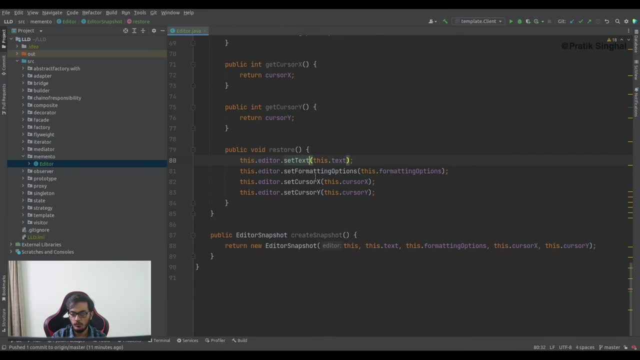 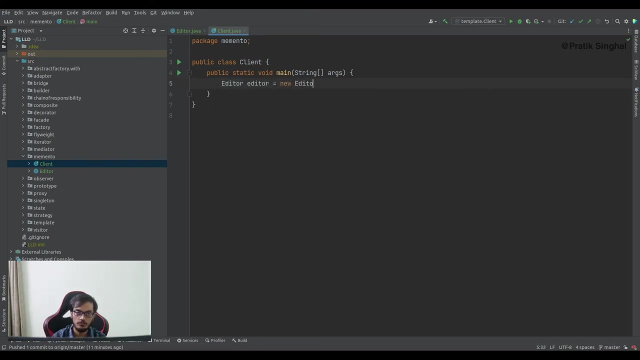 class. there's a restore method, so i can use the restore method to restore it back. so for, For example, let me create a client class now. Now here what I can do. I can create a new editor. I can say: initially, text is just A formatting, options are empty, cursor position is 0, 0. 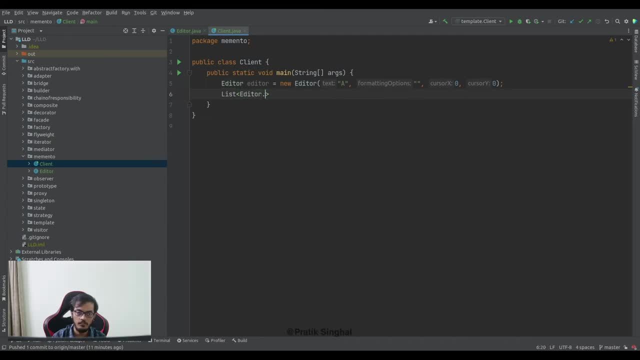 Let's say this is the case and let's say I am maintaining a history of these snapshots in a history list. Now what I am going to do? let's say I have to make some changes in this editor. Let's say I have to change its text to B. So what I will do, I will create a snapshot. 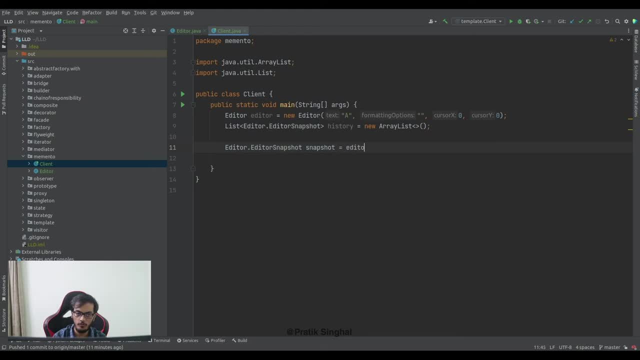 of it: Editoreditorsnapshot. Snapshot will be equal to editorsnapshot. Now, if you see, client class does not have to worry about how to create that snapshot because that responsibility is passed to the editor class itself. So I am using the editor class createSnapshot method. 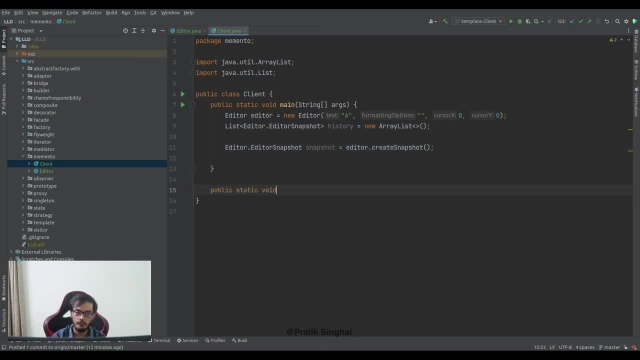 In fact, let me create some helper method here. Public static void: CreateBackup. So this createBackup method will basically create a snapshot, Basically create a backup and return it. It's freeadd, So I am going to create a snapshot of this snapshot and return it. 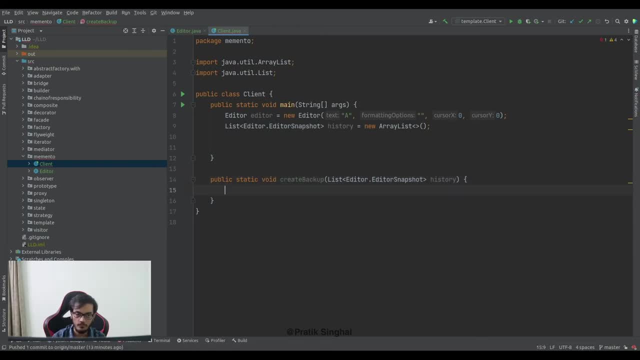 So I am going to create a snapshot of this snapshot and return it. Now I am not going to annotate, So it won't just read out a snapshot. It will say: if here astronautcreate Snapshot. So this is my snapshotcтиров lawyers. 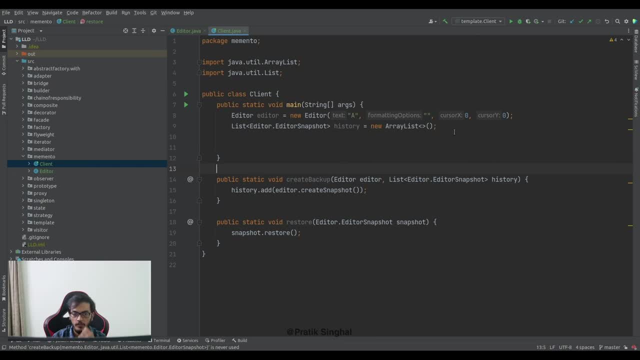 Okay, That's it. So now let's create a snapshot. ok, so right now i have created one initial editor and i have maintained a history array, history list. now let's say i want to make some changes to my editor, i want to change its text. so, before changing the text, i will create a background and i will pass editor. 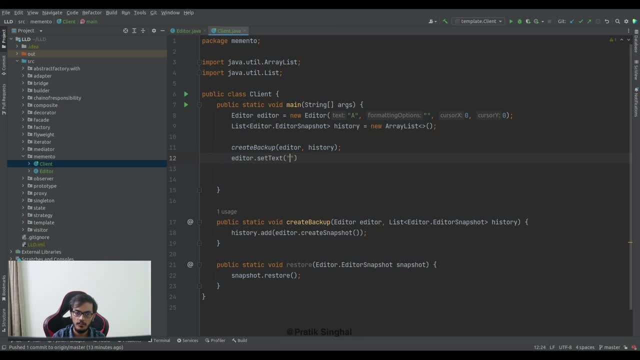 and history as argument, and then i will change the text. editorset text, let's say b. and now if i want to print the text text of editor is editorget text, it will print. text of editor is b. now let's try to restore. so to restore what i will do, i will call the restore function. 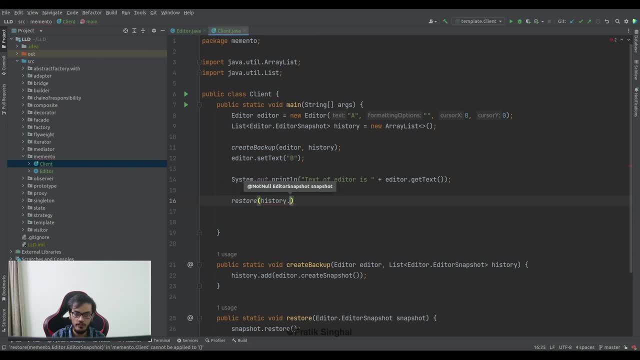 which takes the snapshot as argument, i will say historyget history dot size minus one. basically i am getting the last element from the history list because i want to restore to the latest snapshot right and now. if i say systemoutprintln text of editor after restoration is editorget text, so first it will print.